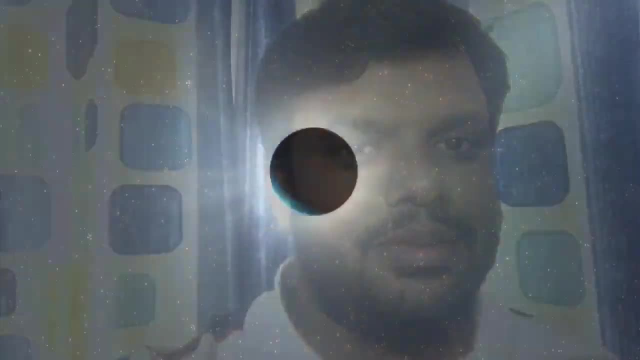 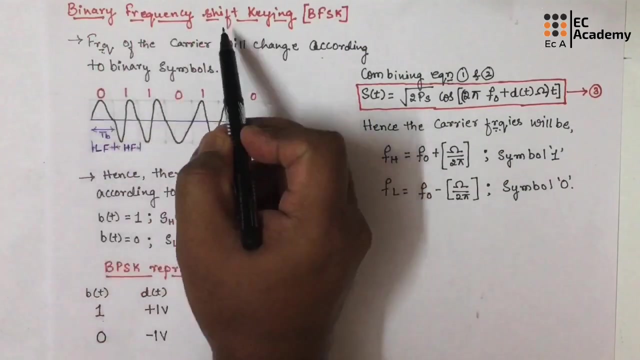 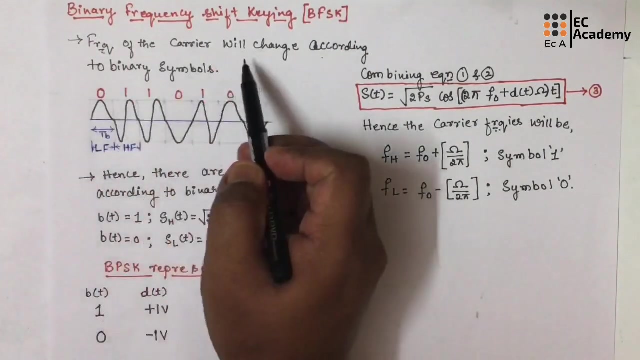 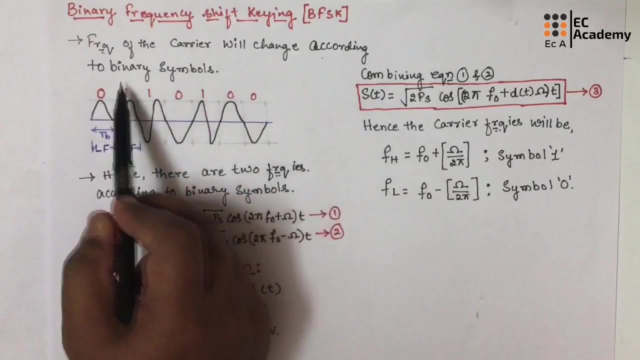 Hello friends, welcome to EC Academy. In this lecture let us understand binary frequency shift keying, which is BF-SK. In this type of modulation, the frequency of the carrier will change according to the binary symbol. So here, the frequency of the carrier will change with respect to the input symbols. 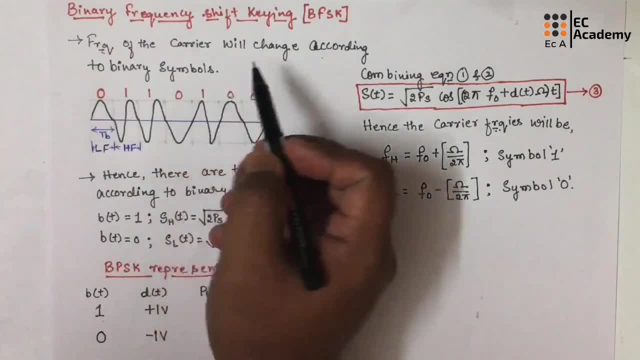 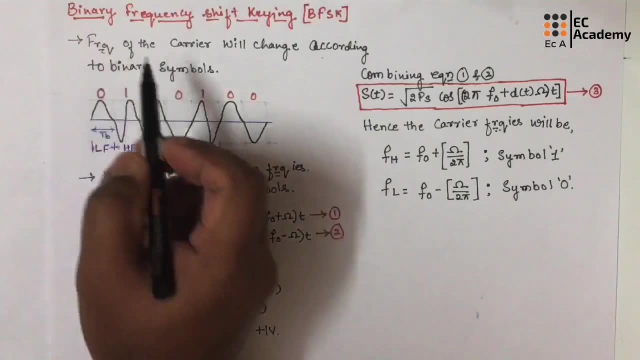 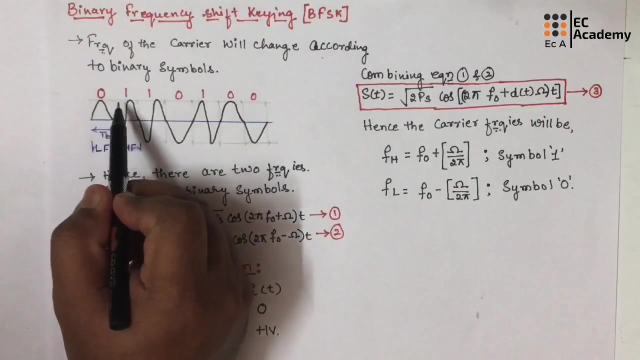 The other parameters of the carrier signal, like phase and amplitude, will not vary. Only frequency of the carrier signal will vary. Such type of modulation is known as binary frequency shift keying. Let us take a binary sequence as an example: 0, 1, 1, 0, 1, 0, 0. 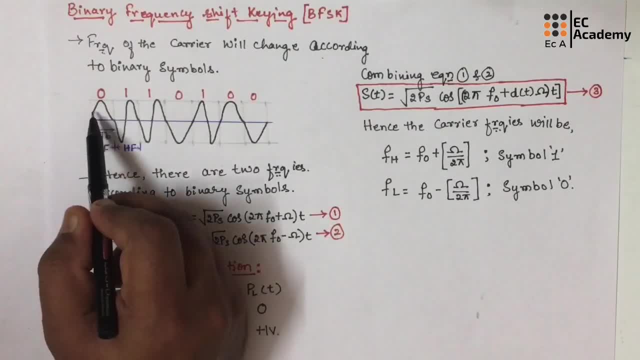 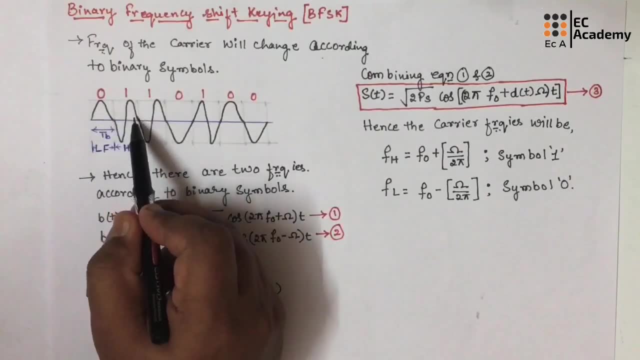 For this sequence. if you observe, the frequency of the carrier signal is low when the symbol is 0. And the frequency of the carrier signal is high when the symbol is 1.. So the frequency will be high when the symbol is 1.. 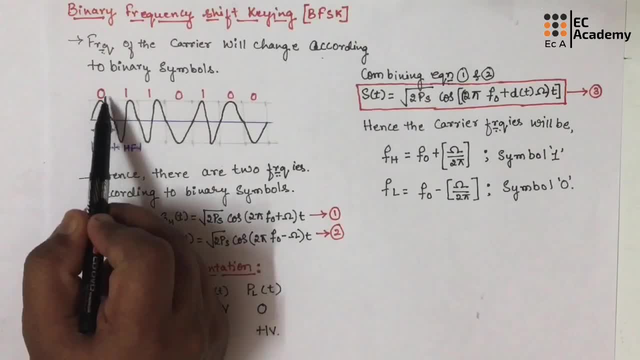 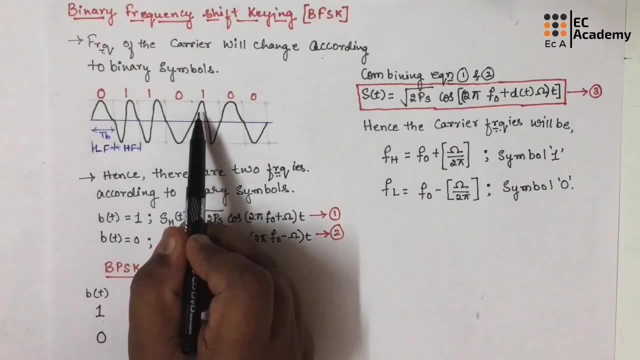 And the frequency of the carrier signal will be low when the symbol is 0. So this process will continue. For 1, the frequency is high. For 0, the frequency is low. Hence we can say there are two frequencies according to the binary symbols. 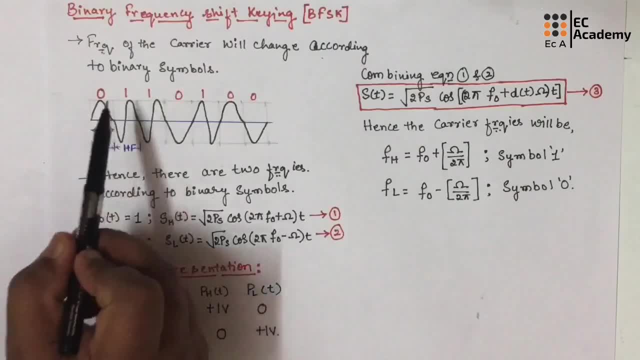 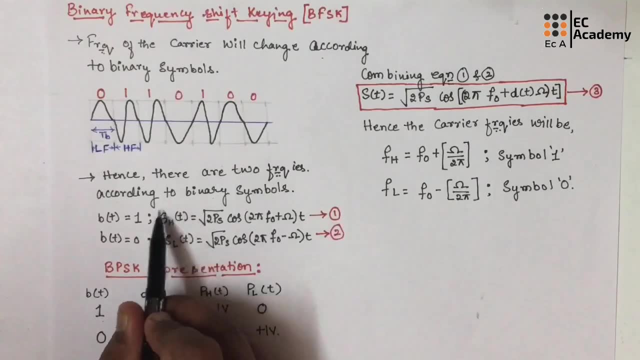 So there is high frequency as well as low frequency, Depending upon The binary symbol. So if the bit is 1,, then the signal will have the high frequency. that can be represented as sh, that is equal to square root of 2ps, cos, 2pi, F0 plus omega into t. 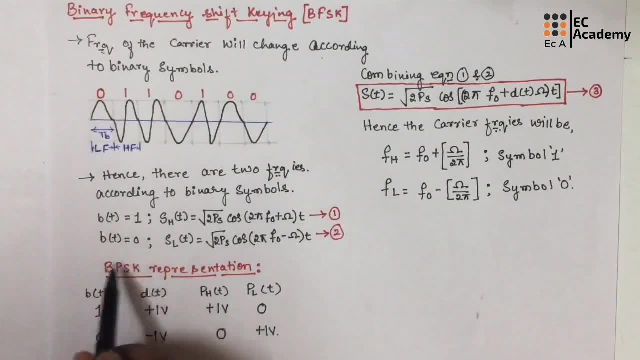 Let us take this as equation number 1.. When the bit is 0,, the signal will have low frequency. that is represented as sl. that will be equal to square root of 2ps, cos, 2pi, F0.. minus 2 and minus 2.. 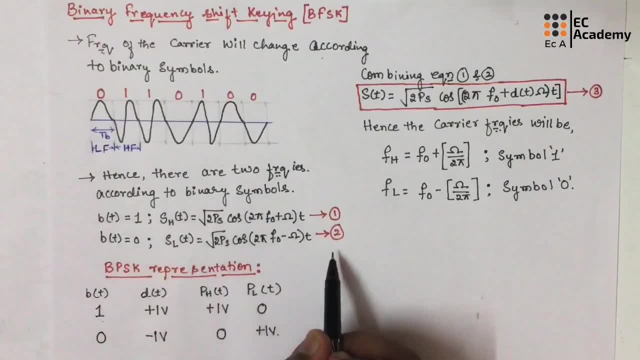 omega into T. Let us take this as equation number 2.. So from these two equations we can identify that the frequency will increase and the frequency will decrease, depending upon omega. So here omega represents the frequency shift. If you can remember, in PSK the phase change was represented by theta. 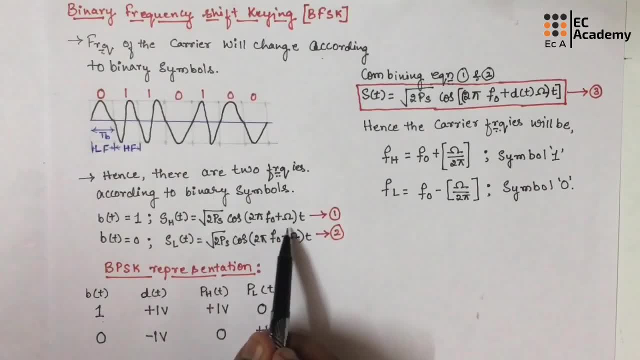 in the same way. the frequency change is represented here as omega. Now let us understand how a BPS K signal is represented. So here B of T is the input sequence, Here D of T is the representation of input sequence, and here we are having pH of T and PL of T. These two will be considered when we 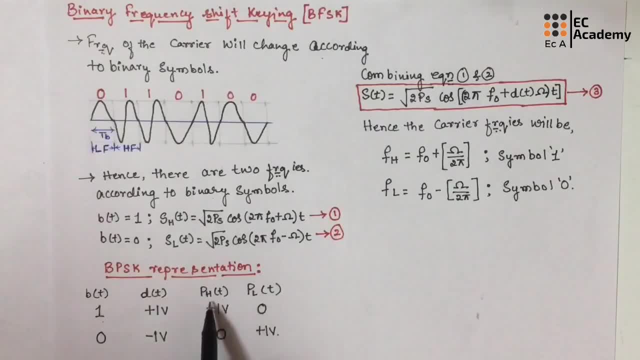 are transmitting the signal For time being, just remember this- as high frequency and low frequency. When the input bit is 1, then D of T is considered as plus 1.. The high frequency is represented by plus 1 volt And the low frequency is represented as 0, because for 1 we know there is high frequency When the 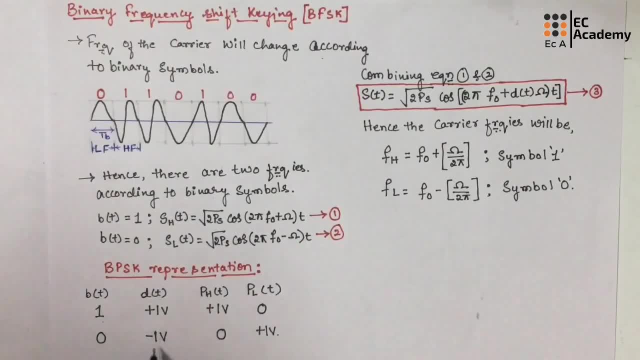 bit is 0. D of T is represented as minus 1 volt. So high frequency is represented as 0 and low frequency is represented as plus 1 volt, because 0 represents low frequency. So if you observe here, pH of T and PL of T are complementary to each other. When pH of T is 1, PL of T will be 0. 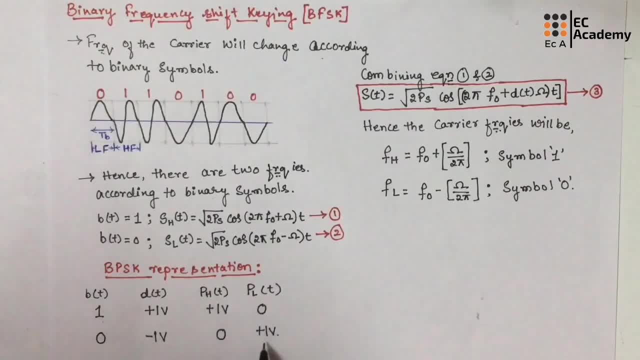 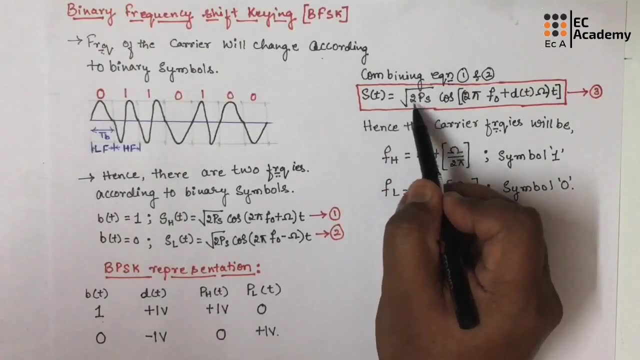 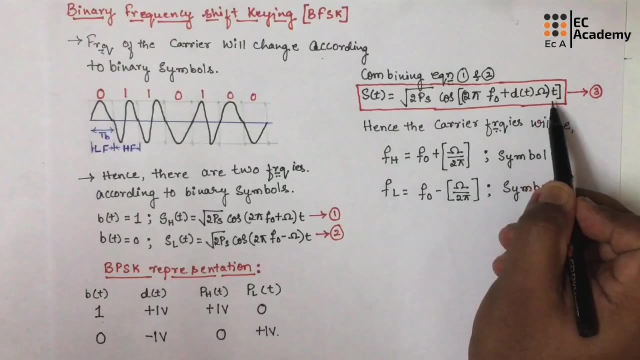 And when pH of T is 0, PL of T will be 1.. Now let us combine equation 1 and 2 and write a signal which is S of T is equal to SW2PS, cos Do into omega T. So let us call this as equation number 3.. In this equation, if we put D, 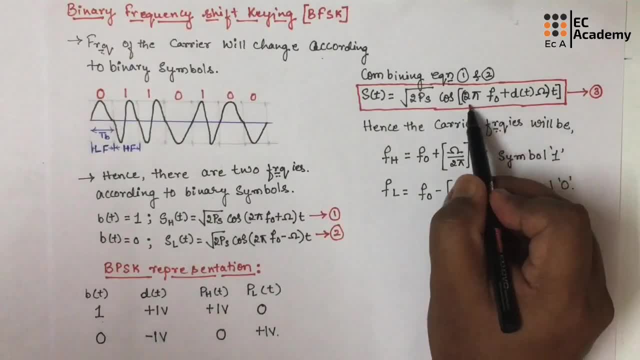 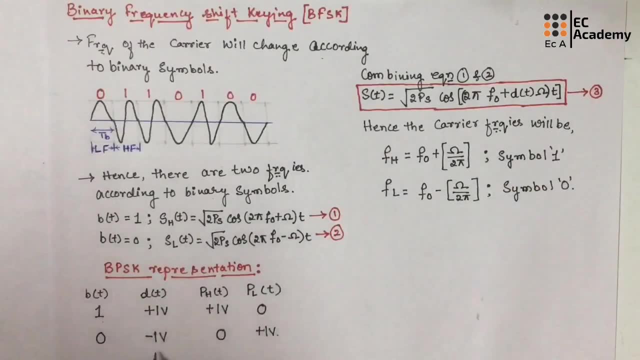 of T is equal to plus one, So the equation will become 2πF0 plus omega 들어가, which means this signal will represent bit 1.. When we put d of t is equal to minus 1, the equation will become 2 pi f naught minus omega, which means this sequence will represent bit 0. Hence we can. 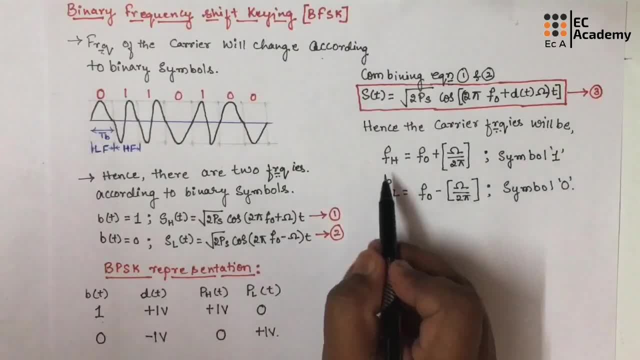 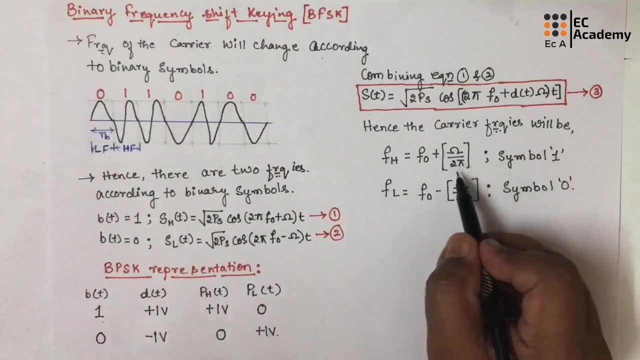 say the carrier. frequencies will be high frequency as well as low frequency. High frequency can be represented as f? naught plus omega, divided by 2 pi, when the symbol 1 is transmitted, and low frequency is represented as f? naught minus omega divided by 2 pi when symbol 0 is transmitted. 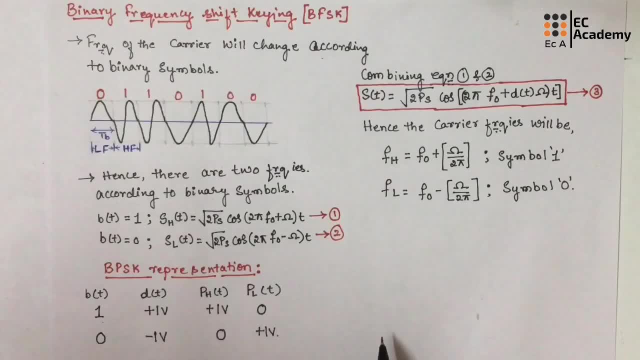 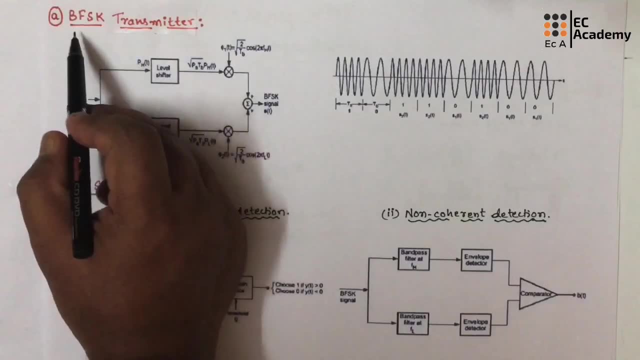 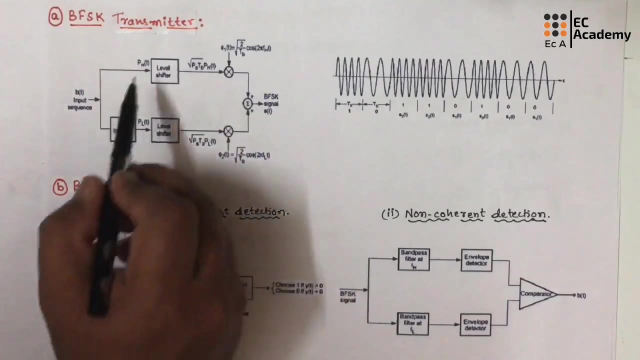 So this is about the introduction of BFSK signal. Now let us understand the generation and reception of BFSK signal. First, let us understand BFSK transmitter. The block diagram of BFSK transmitter is shown in this figure. Here, pH of t is same as B of t and PL of t is inverted version of B of t. 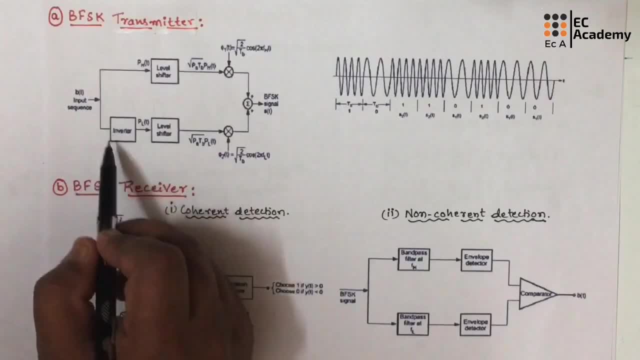 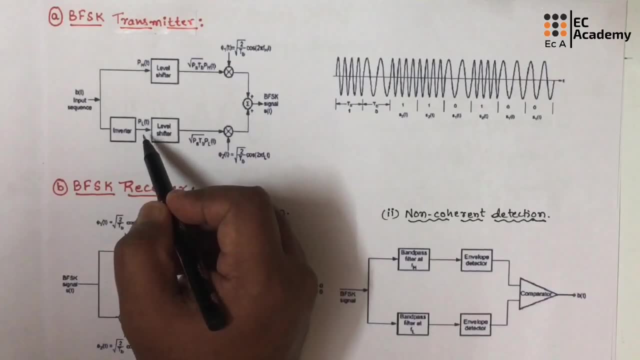 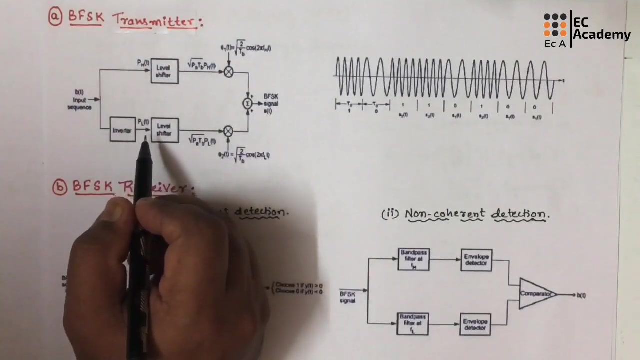 That is why the inverter is added after B of t to get PL of t. Here pH of t and PL of t are unipolar signals. So here pH of t represents the high frequency signal, PL of t represents the low frequency signal, The level shifter. 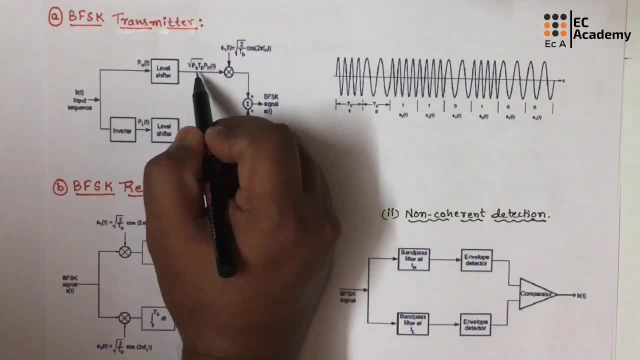 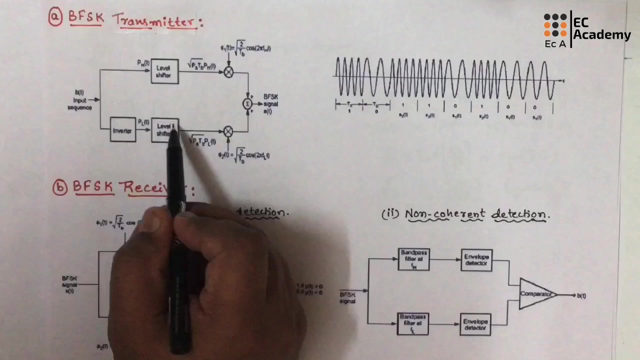 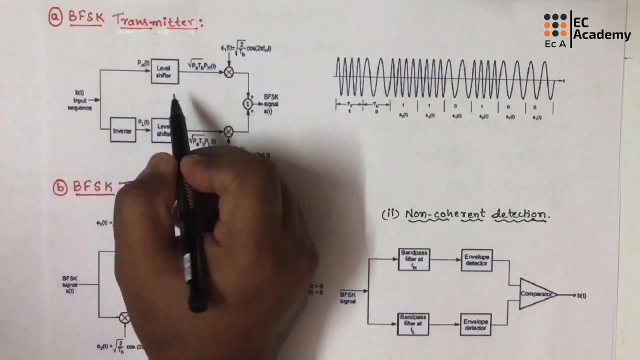 now what we understand, into which the signalTV exception. we can also explain it in two ways. First, byetas: if the output of the level shifters is PL, Then if the input of the signal is 1, then input of the level shifters will be Time S. 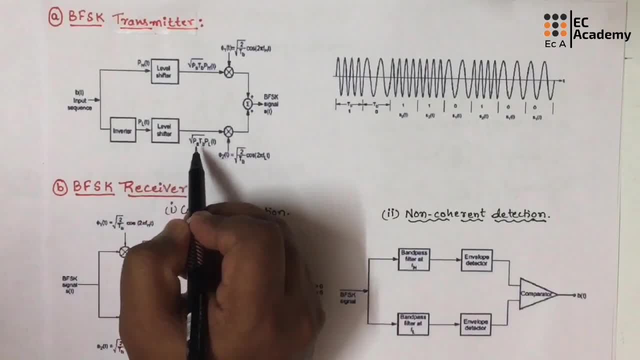 Plus 1 Volts And then themoments approaches 1 V to srps into2Pb and the 0 V will be unaffected is 0, the output of the level shifter will be 0.. After level shifter there is: 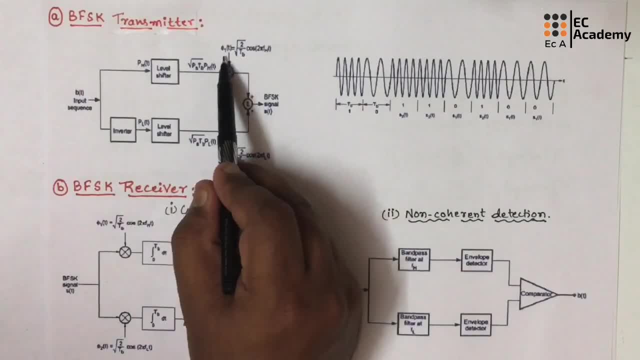 product modulator, Two carrier signals, 5: 1 of t and 5: 2 of t, are used, and these two signals are orthogonal to each other. The adder will add these two signals to produce BSFK signal. Here you need to remember the output of the multiplier. 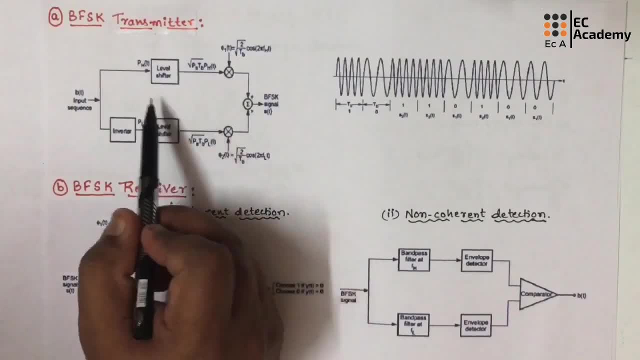 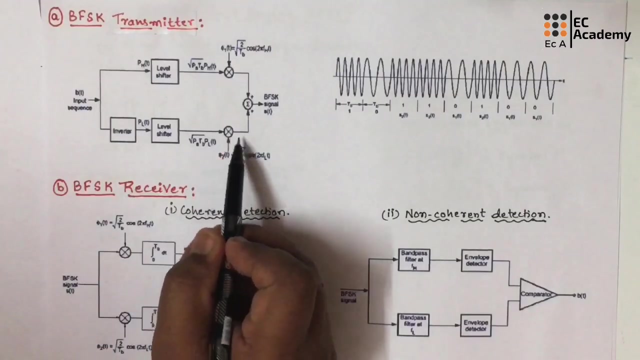 are not possible at the same time because PH of t and PL of t are complementary to each other. For example, if PH of t is 1, the output will be only from the upper modulator and the output of the lower modulator will be. 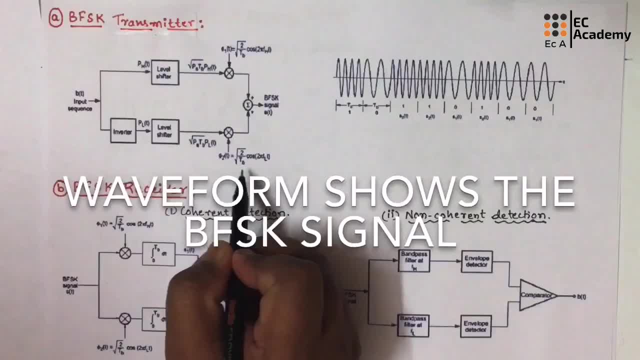 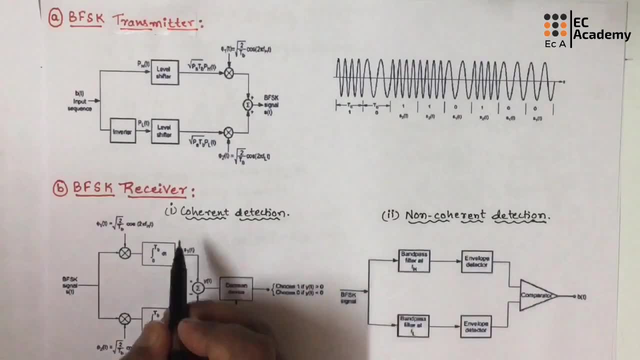 zero. So this is about the transmitter. Now let us understand BFSK receiver. In BFSK receiver there are two types. First one is coherent detection and second one is non-coherent detection. In coherent detection we know that at the receiver end there will be a local carrier that will tune with the carrier of the transmitter. 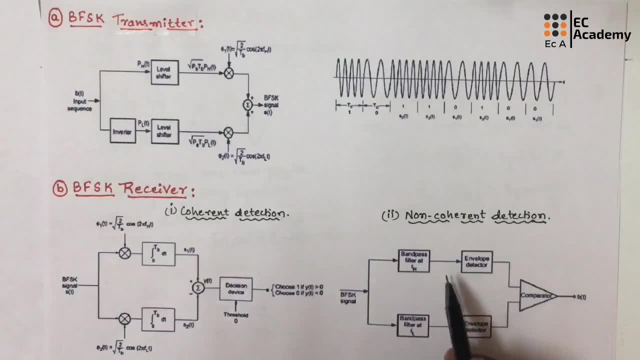 In non-coherent detection, there will be no local carriers at the receiver end. First, let us understand the coherent detection of BFSK signal. This figure shows the block diagram of coherent BFSK receiver. There are two correlators, which consist of multiplier and integrator. 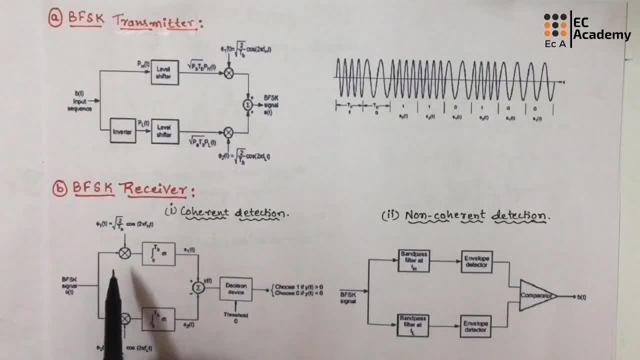 This correlator provides local generated carriers as phi 1 of t and phi 2 of d. Output of the multiplier is given as input to the integrator that will produce the output: s1 of t at the upper integrator and s2 of t at the lower integrator If the transmitted frequency is fs. 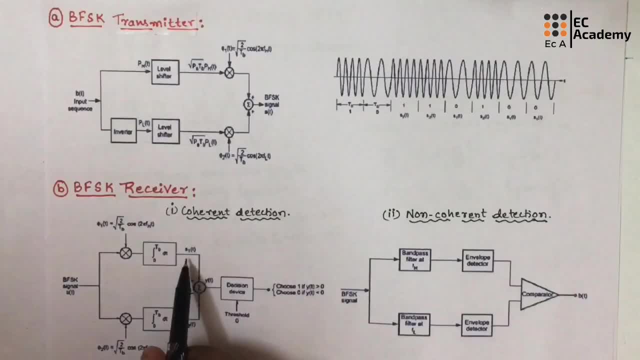 which is high frequency, then the output s1 of t will be greater than s2 of t. and if the transmitted frequency is fl, which is low frequency, then the output s2 of t will be greater than s1 of t. If s1 of t is greater than s2 of t, we will get at the adder y of t. 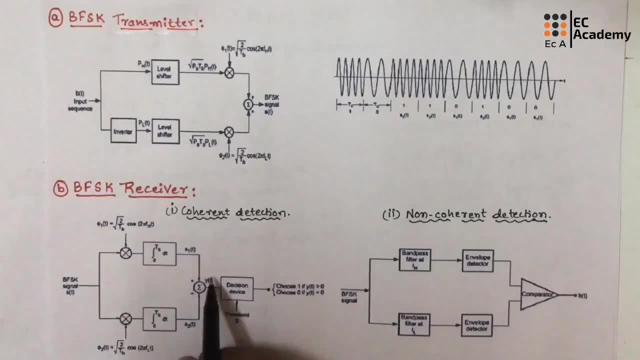 which is greater than 0.. If y of t is greater than 0, then the decision making device will choose bit 1 as transmitted bit. If s2 of t is greater than s1 of t, at that case y of t will be less. 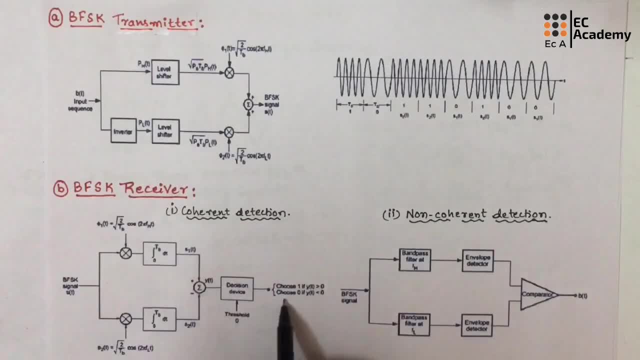 than 0.. At that case, decision making device will choose bit 0 as transmitted bit. So this is about the coherent detection In non-coherent detection. this block diagram shows the non-coherent BFSK receiver. The receiver consists of two bandpass filters: One bandpass filter. 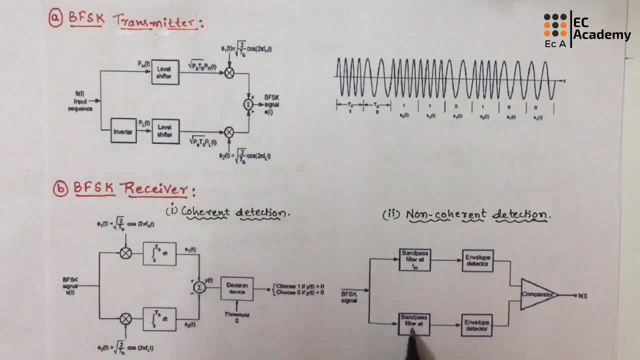 with single bandpass filter is the non-coherent BFSK receiver. The receiver consists of two center frequency FH and another bandpass filter with center frequency FL. We know that FH minus FL is equal to 2FB. Therefore the output of the filters do not overlap The bandpass filter. 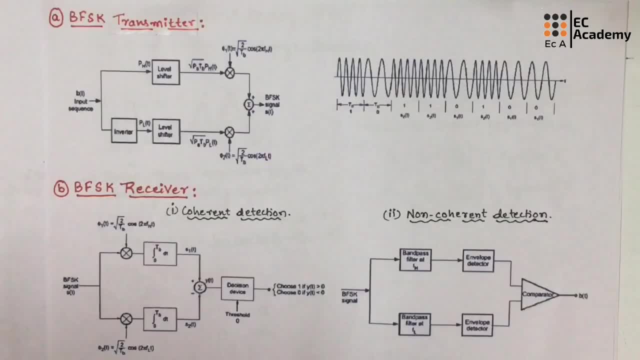 pass their corresponding main lobes without much of a distortion, Since the signals are not overlapped. the output of the filter is applied to the envelope detectors. The output of envelope detector are compared by a comparator, which is a unipolar comparator. Hence output of the comparator will be the bit sequence B of t. So this is about non-coherent.